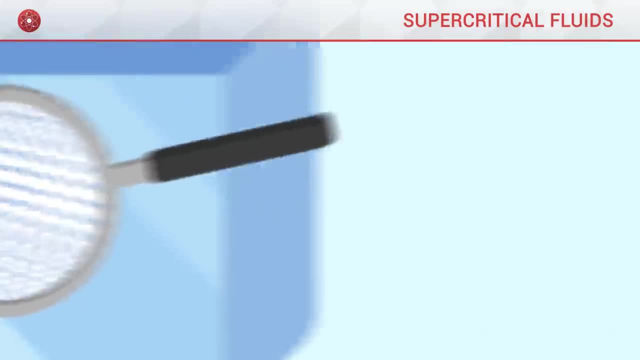 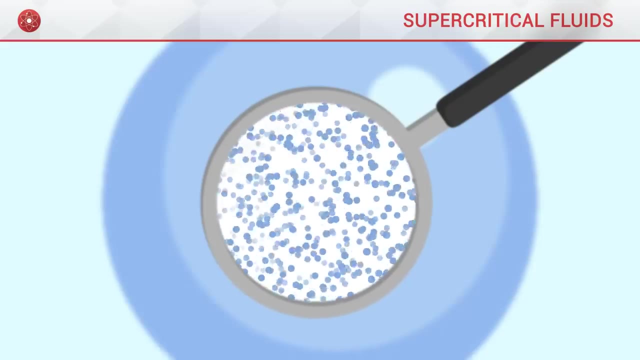 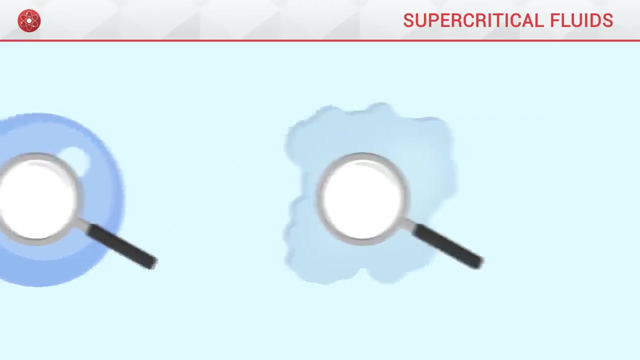 structure because they are strongly bound. In a liquid, molecules are more loosely bound. They are free to move around, but they maintain a certain cohesion. A liquid can be deformed, but it conserves a certain volume. This contrasts with gases, in which molecules are free to move. 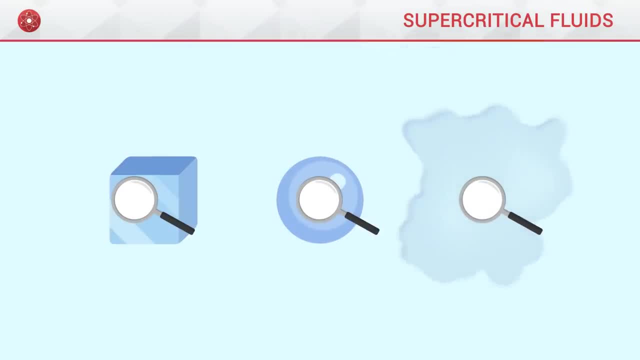 around and eventually take up the entire volume in which they are formed, Depending on the temperature and pressure of the environment. a body will naturally be in one of these three states, For instance, at atmospheric pressure and in the range between 0 and 100. 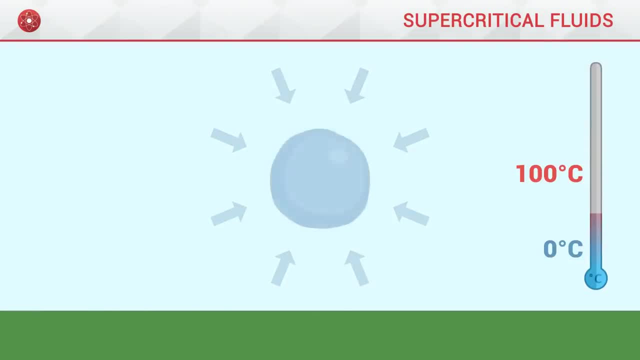 degrees Celsius, water is naturally liquid. These are the conditions of our atmosphere and explains why liquid water can be found on the planet. If the temperature were 200 degrees Celsius, keeping pressure constant, water would be found as a gas water vapour. 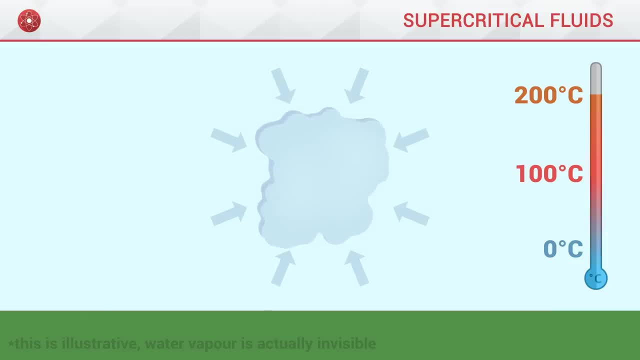 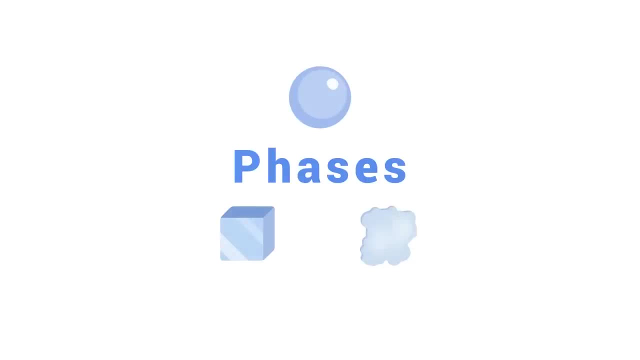 In order to model the conditions required for the presence of each of the three states of matter, we can draw a phase diagram. Such a diagram represents the phase of water, in other words, the state in which it occurs, naturally for different values of pressure and temperature. 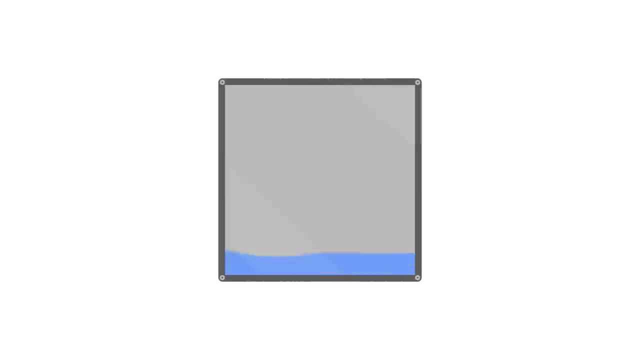 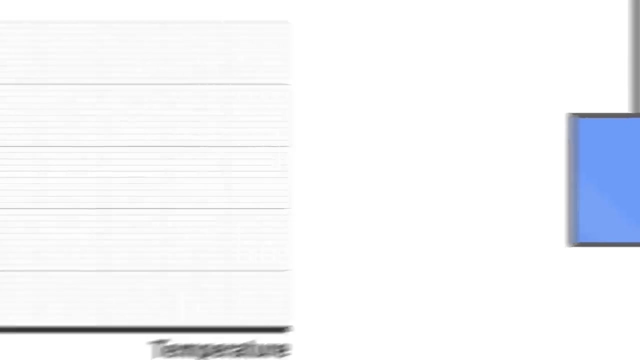 We start by taking a tightly sealed container into which we will pour water. The temperature in the container can be adjusted through heating or cooling and the pressure can be altered by pressing or pulling a piston. To fill in the diagram, we will use three colours. We choose to use grey for gas light. 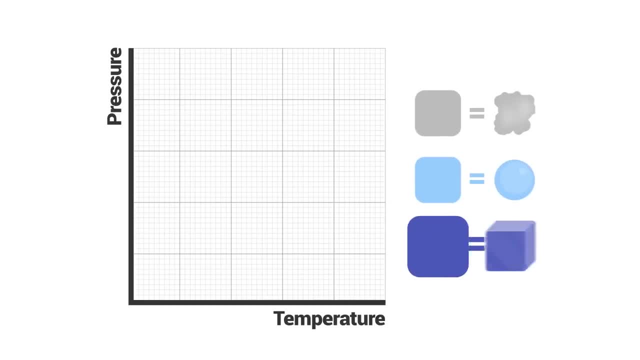 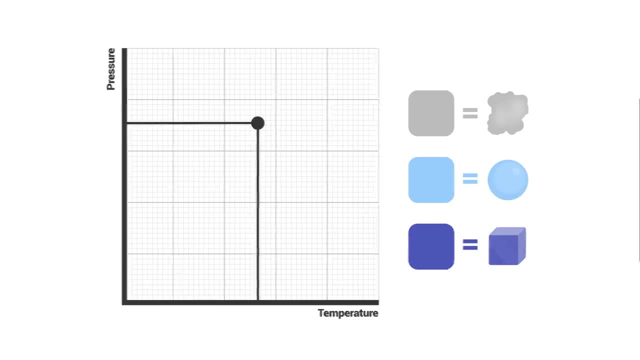 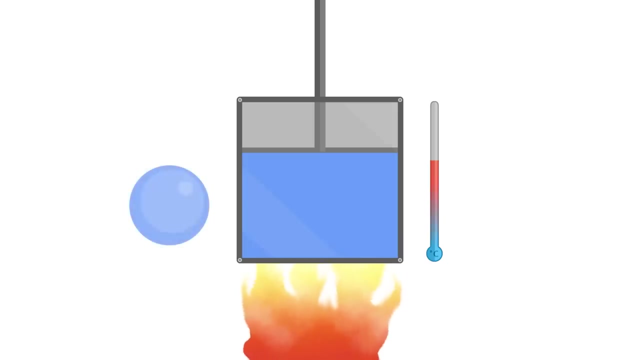 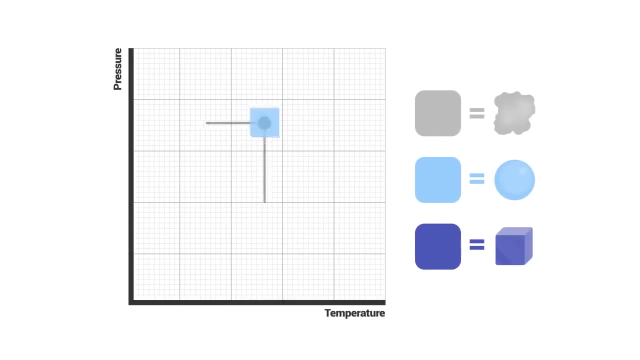 blue for liquid and dark blue for solid. Each point of the diagram corresponds to a unique temperature-pressure combination which we will replicate inside the container. We can observe which phase the water inside the container is in and draw a small square on the diagram with the corresponding colour, By repeating this process for multiple values. 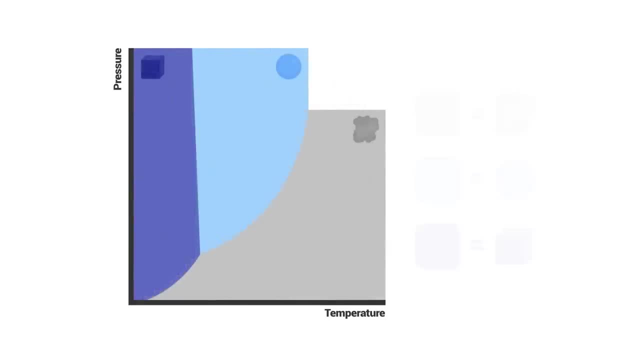 we finally obtain a map on which three zones appear. If a given pressure-temperature pair lands inside one of these zones, for example in the dark blue zone, we can see that the pressure-pressure combination is not the same as the pressure-pressure combination. 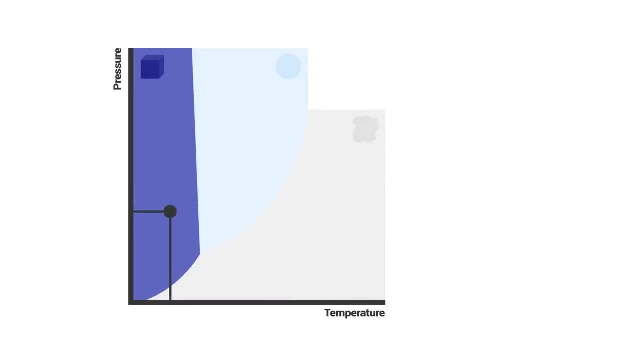 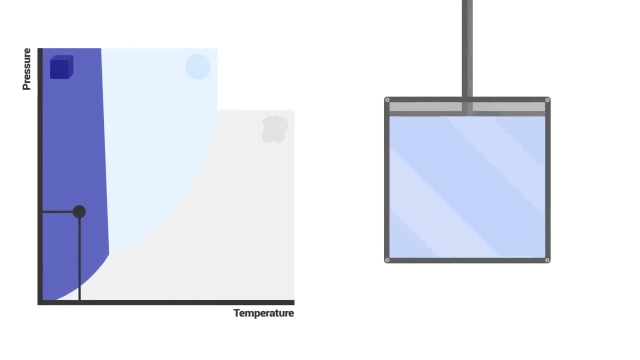 The pressure-pressure combination is the same as the pressure-pressure combination, but the pressure-pressure combination is different. The pressure-pressure combination is different. This means that under these specific conditions, water is naturally in a solid state. One of the first things that stands out is the fact that the three zones have precise 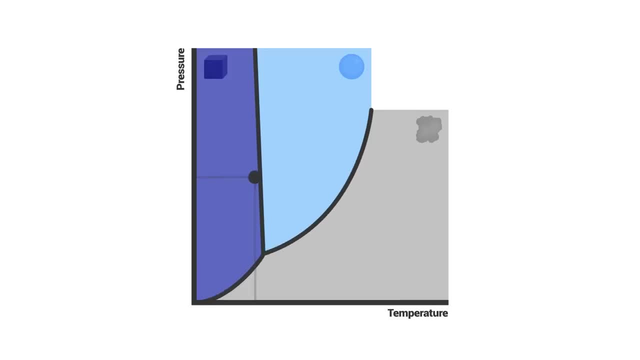 boundaries, When we are at the limit between two zones, the two states on either side of the boundary can coexist simultaneously in a stable way. For instance, when we heat up an ice cube, we see Bilcarra I below and below the ice cube. Biohazard, cold war here. 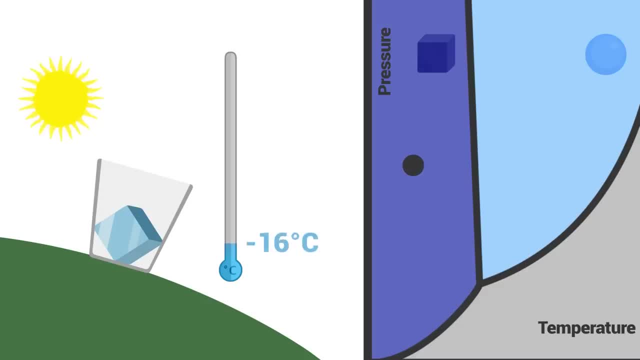 is also a veryak totality of a tried A vector. S? 나 means under the water in any地, losing the 나도, the relationship societ, Maybe Biraz, when we are at the limit of the two zones o temperature. it gradually moves to the right of the diagram as its temperature increases. 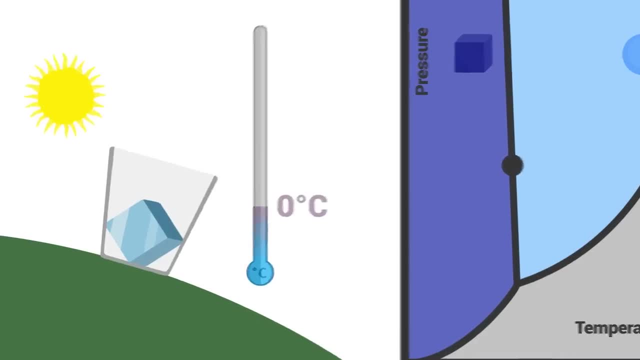 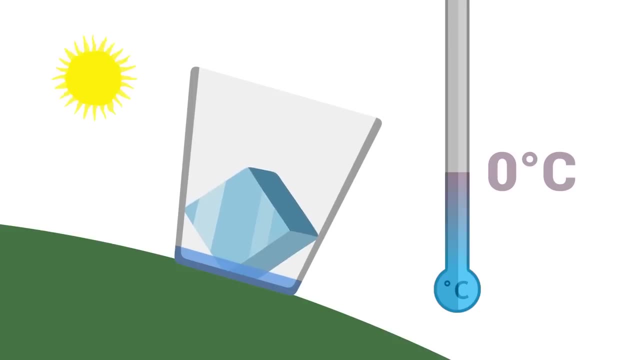 When we reach the limit of the solid zone, a temperature of 0°C, the very first drops of liquid water appear. Gradually, the ice cube melts. while remaining at the same temperature, The energy supplied through heating no longer changes its temperature, but instead causes. 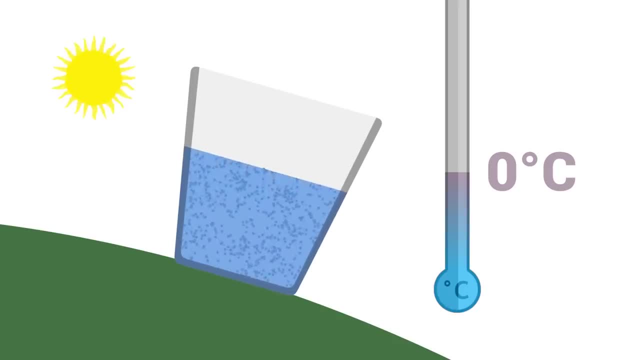 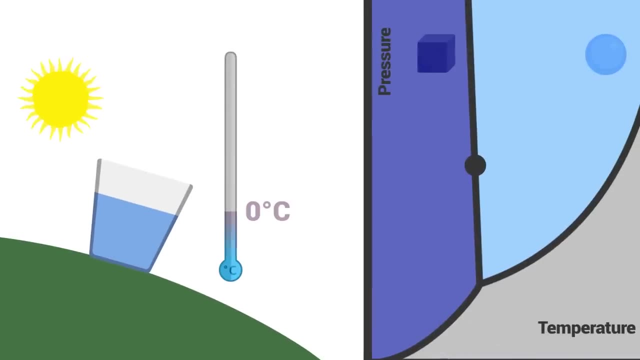 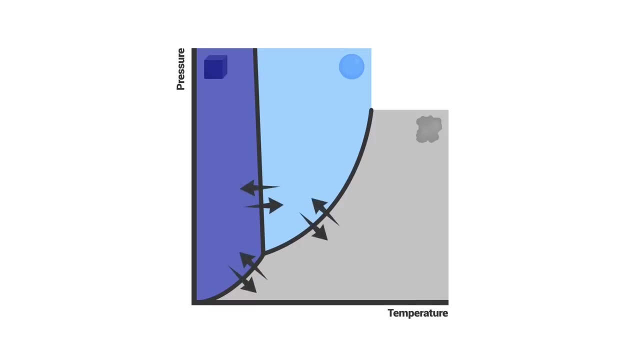 it to melt, to rearrange its molecules on a microscopic scale. Once the ice cube is entirely melted, its temperature will start to rise again, signalling a movement into the zone of the diagram corresponding to the liquid state. We have performed a phase transition, going from one state of matter to another, by crossing one of these boundary. 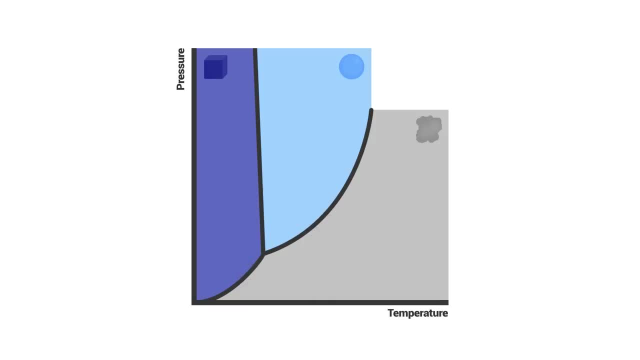 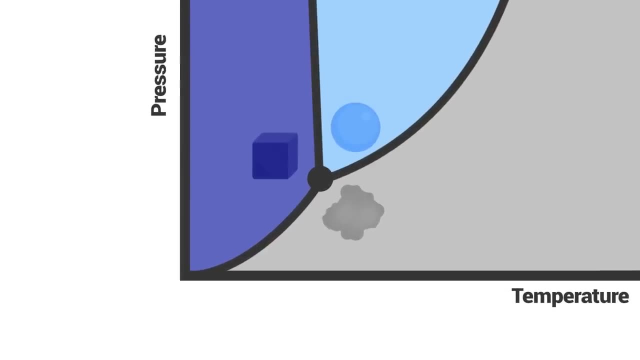 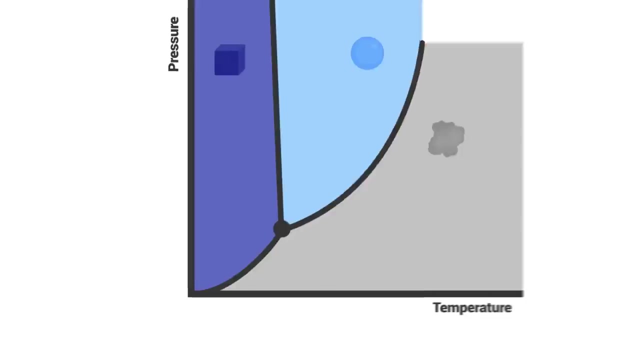 curves. Another point which deserves mentioning is that there exists a point in the diagram where the ice cube is completely melted and the temperature is 0°C. This is the point at which the three zones touch. This is a point of contact between each possible state of matter: solid, liquid and gas. Under these specific conditions of 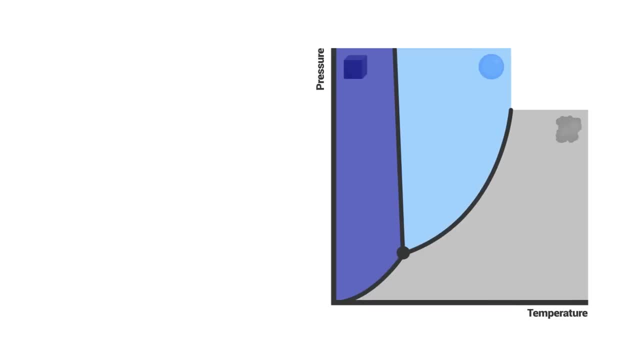 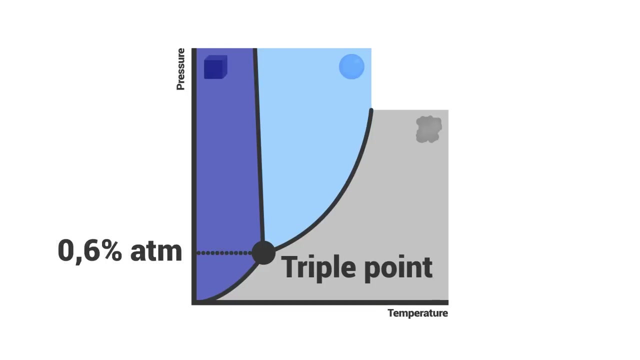 temperature and pressure. it is thus possible for water to coexist in a solid, liquid and gas form all at once. This peculiar setting is called the triple point. For water, this triple point corresponds to a pressure of 0°C, The temperature is 0.6% of an atmosphere and a temperature of one hundredth of a degree. 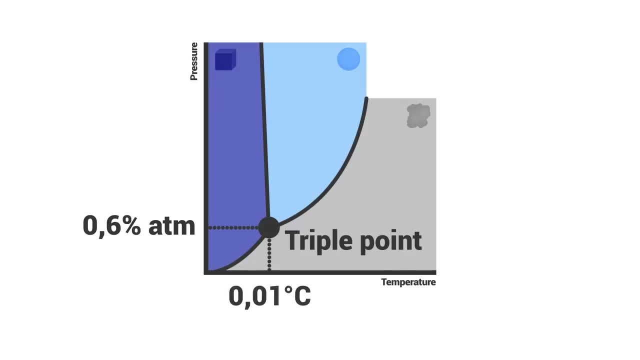 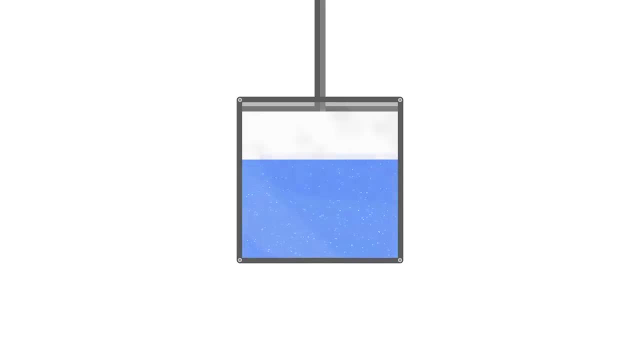 Celsius, Conditions that do not occur naturally on Earth, but which we can create in a lab, allowing us to surprisingly boil water while some of it is simultaneously frozen. Coming back to the phase diagram, what interests us most is the fact that the curve separating 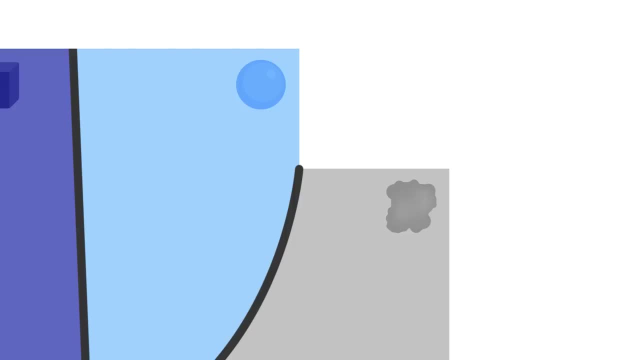 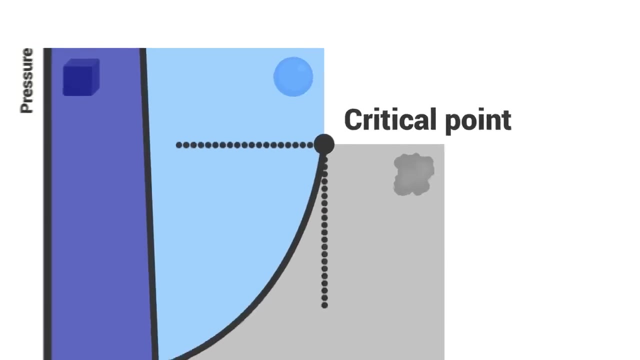 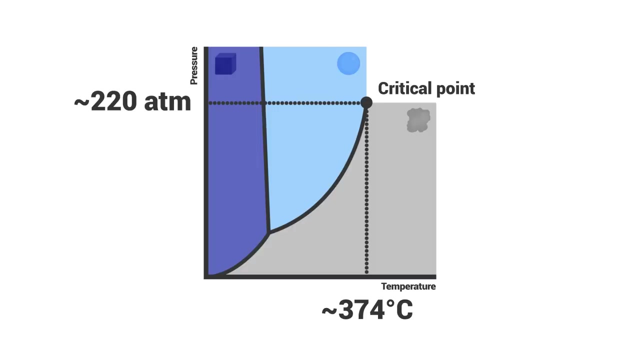 liquid and gas seems to stop abruptly. This specific point is the point at which the liquid stops. The point where the curve stops is the critical point. It corresponds to a very high temperature and pressure combination, conditions that do not occur naturally on Earth, but which can be reproduced in a laboratory. 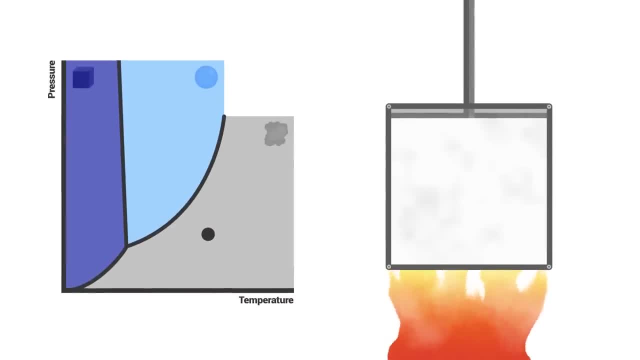 Let's take our water container and adjust its pressure and temperature in order to lie on this curve. As we have seen, at the boundary between the two zones, water appears simultaneously in two different states. This is the point where the curve stops- and the temperature. 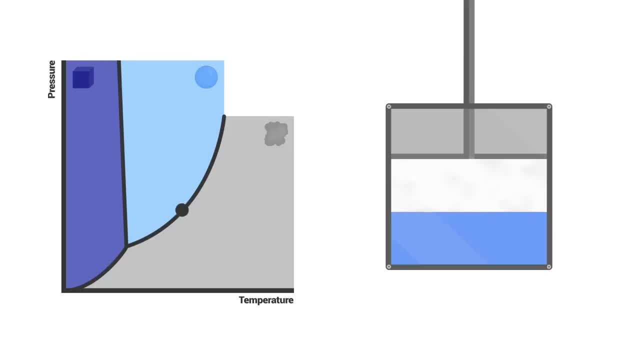 stays the same. This is the point where the curve stops and the temperature stays the same. Inside the container, we see a separation between liquid water and water vapour. Let's now gradually heat and compress the container so that we approach the critical. 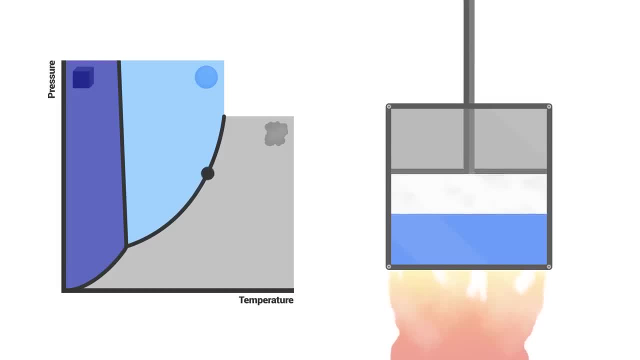 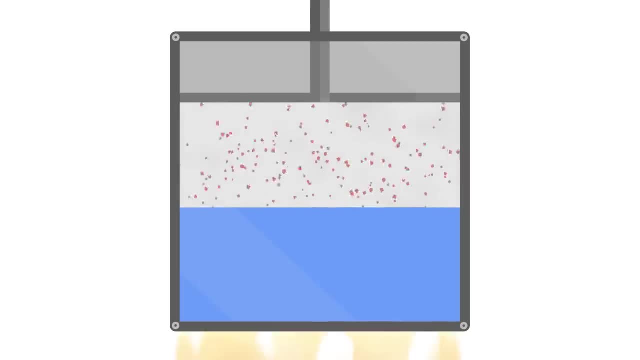 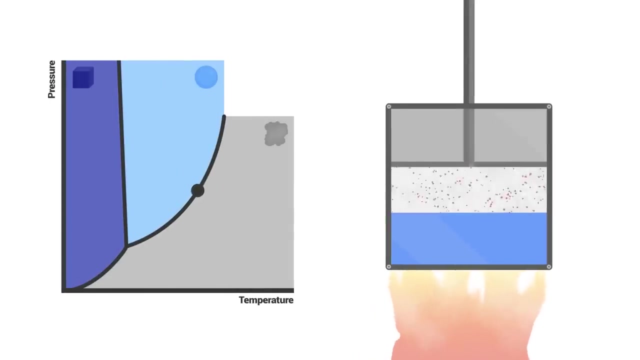 point while remaining on the curve. As pressure increases, the water molecules in the gas are strongly compressed. They come closer together and take up less space. The vapour becomes more dense. On the other hand, increasing the temperature forces the molecules in the liquid to vibrate. 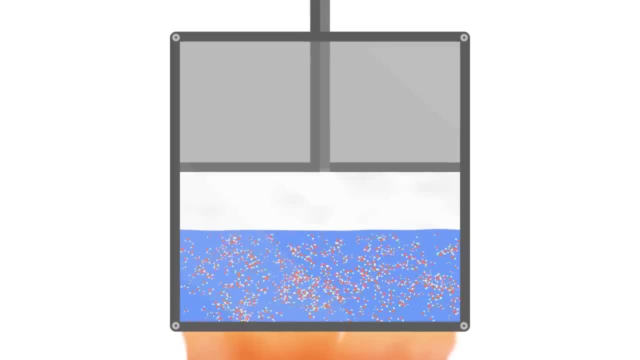 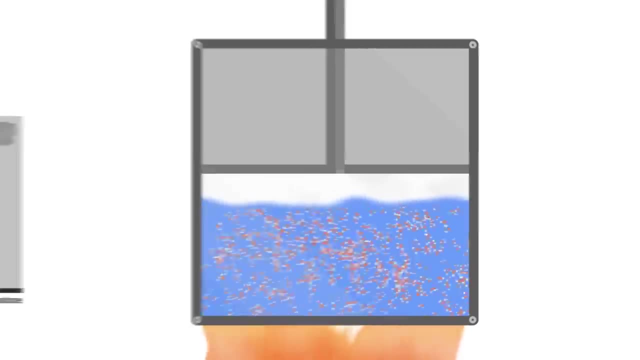 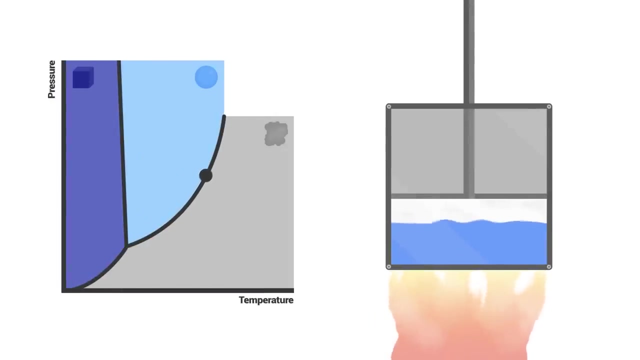 more and more. In this way, the molecules are less bound to each other and their increasing agitation makes them occupy more space. The liquid water becomes less dense Gradually. the separation between the liquid and the vapour becomes less dense. The liquid water becomes less dense Gradually. the separation between the liquid and the 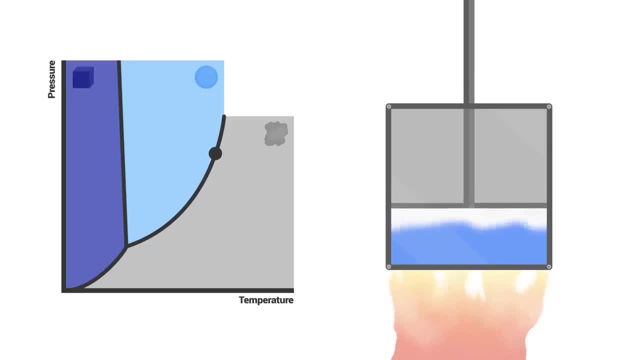 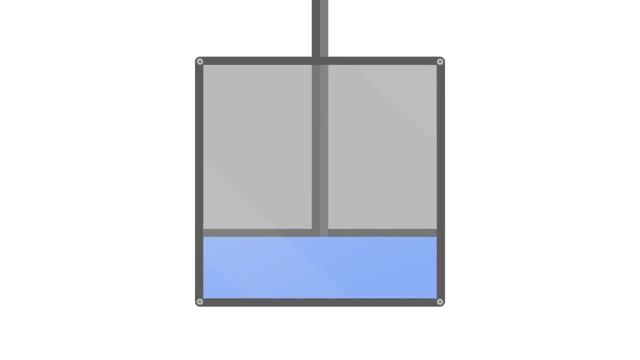 vapour becomes less and less visible. Suddenly, the density of the liquid, which decreases, and that of the gas, which increases, reach the same value. From that moment on, the two phases are no longer distinct. The liquid and the gas in the container have exactly the same density. 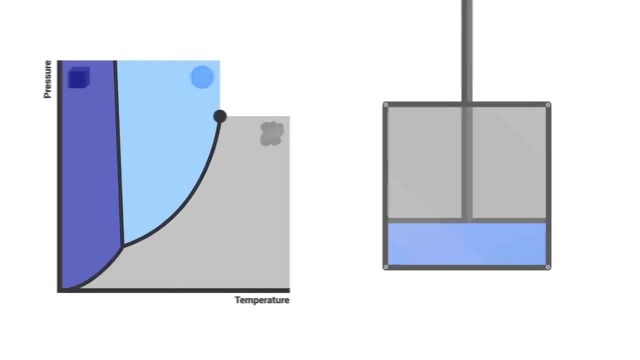 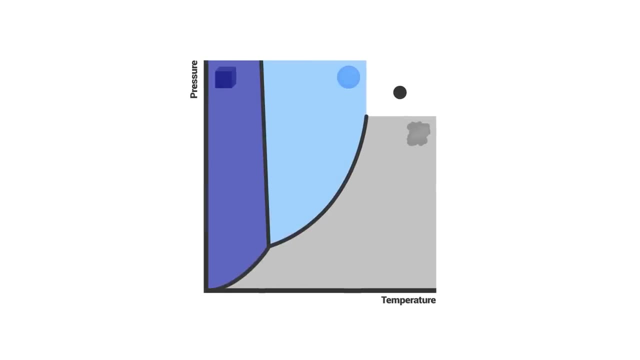 We obtain a sort of homogeneous mixture of liquid and gas. We have reached the critical point. Beyond this point, it is impossible to distinguish the gas from the liquid. The two phases have merged into one. The state of this water is neither liquid nor gas. 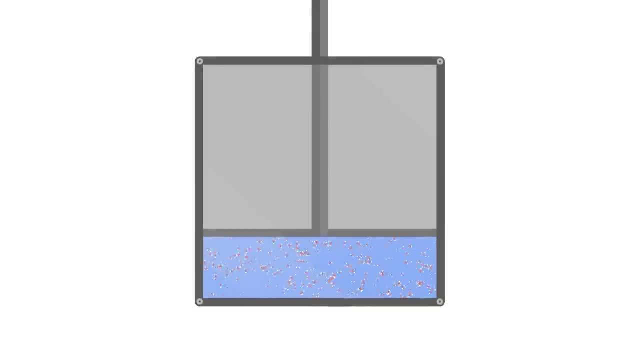 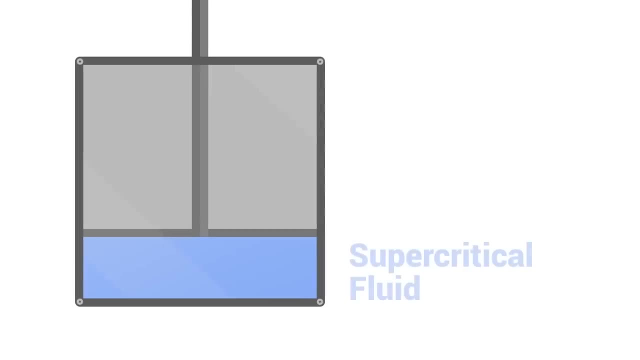 Its behaviour is fairly similar to that of a gas, but it also exhibits interesting properties that are usually attributed to liquids. We call this state a supercritical fluid. It is interesting to note that, unlike the solid state, liquid and gas are not independent. 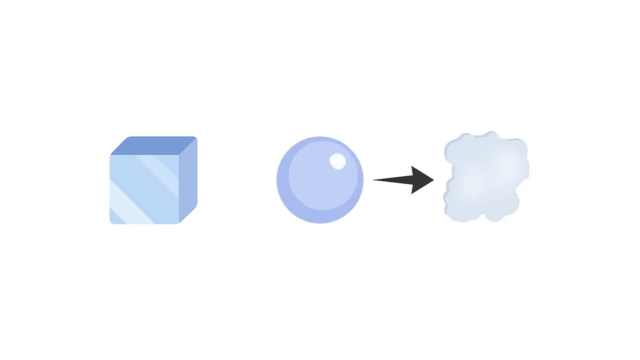 Although it is possible to go from liquid to gas by transition by boiling water, it is also possible to go from liquid to gas without any such transition. To do this, we simply adjust the temperature and pressure in our container in order to bypass the boundary between the two states. 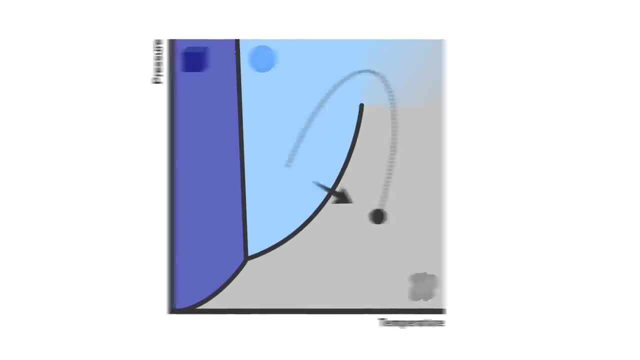 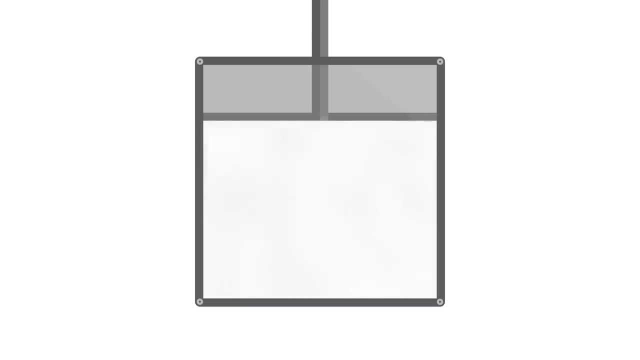 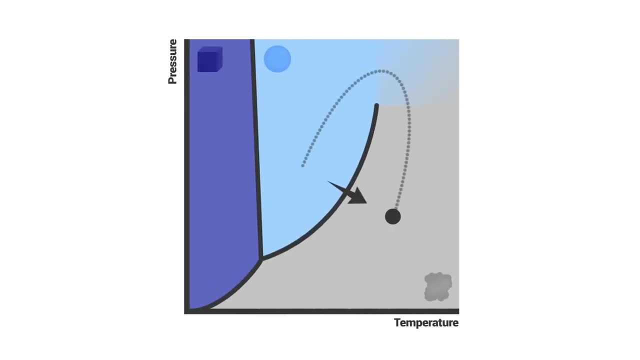 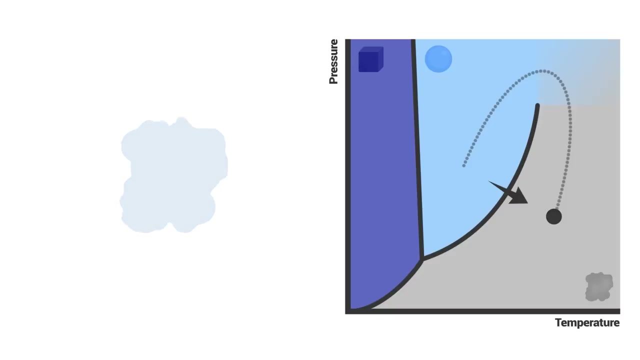 3. We start with a liquid and by making it a supercritical fluid, we can transform it into a gas. This experiment is astonishing to observe. It is very unusual to witness a liquid becoming a gas without any visible transition. Taking our supercritical fluid once again, we can observe a surprising phenomenon as 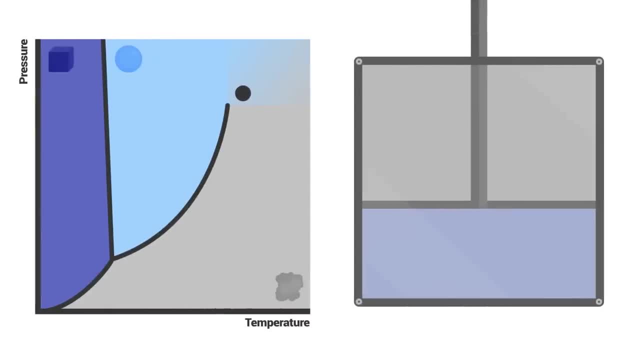 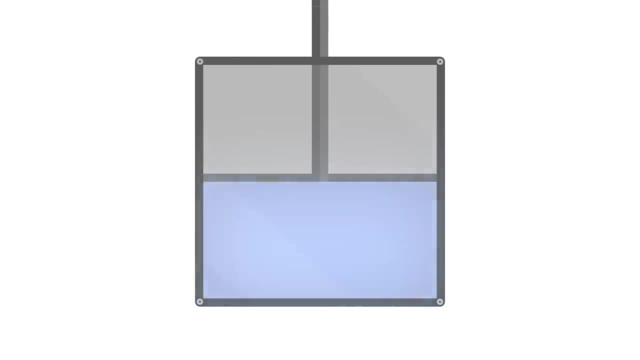 we approach the critical point. As the fluid reaches this point, it spontaneously begins to scatter light. This is called critical opalescence. It is due to the refraction of light within the fluid. Light rays slow down depending on the fluid's density. 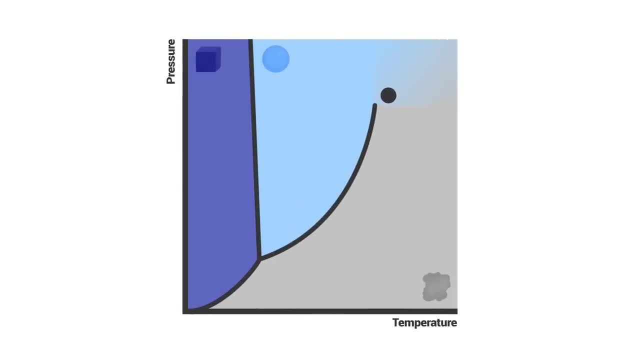 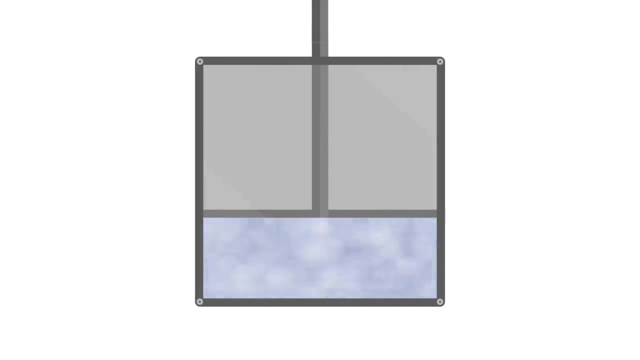 As it approaches the critical point, the fluid has to split into a liquid and a gas, But just before this happens, it hesitates between one state and the other. This is called critical opalescence 3. These hesitations within the fluid lead to strong density fluctuations which scatter. 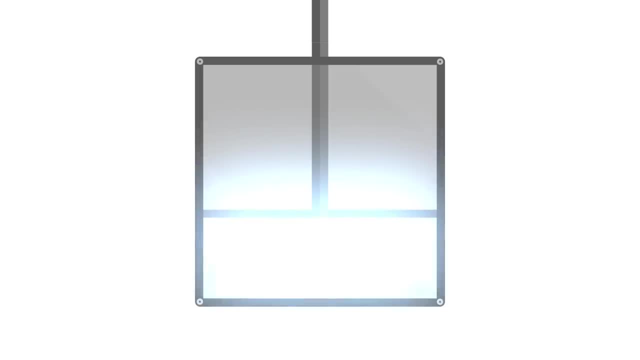 light, In the same way that our atmosphere scatters sunlight, giving the sky its colour In our daily lives, supercritical fluids have many applications. Their properties are very interesting. For instance, although they behave mainly like a gas, we can use them as solvents. 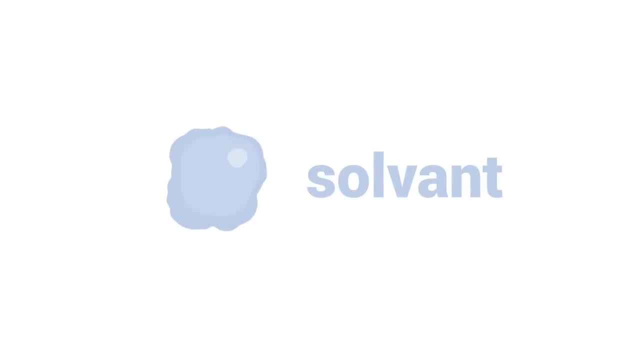 they can serve to extract certain substances. supercritical carbon dioxide is widely used to extract flavors from plants, nicotine from tobacco or even caffeine from coffee. a major advantage of supercritical co2 is that, unlike liquid solvents, it is non-toxic and relatively easy to use with. 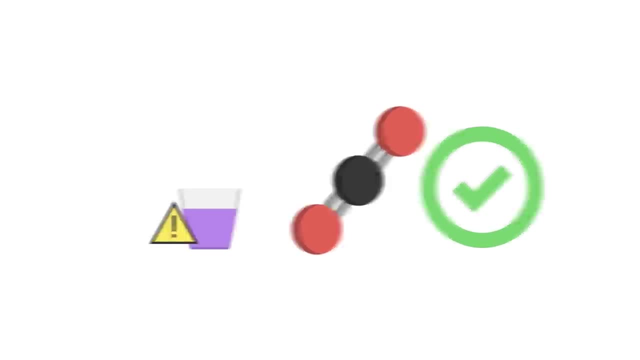 a very high extraction power. in its supercritical form, water is also a very good solvent. it is useful for destroying organic waste without releasing harmful gases as opposed to burning it. supercritical fluids have a multitude of diverse practical applications, such as fuel production, refrigeration or even microbial protection. 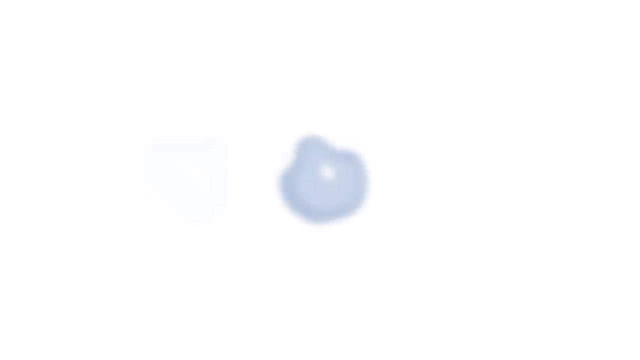 to conclude, the critical fluid is a state of matter in its own right. above a certain pressure and temperature point, liquid and gas seem to merge, forming a single homogeneous state with both gas and liquid-like properties on earth. temperature and pressure are too low to allow for such. 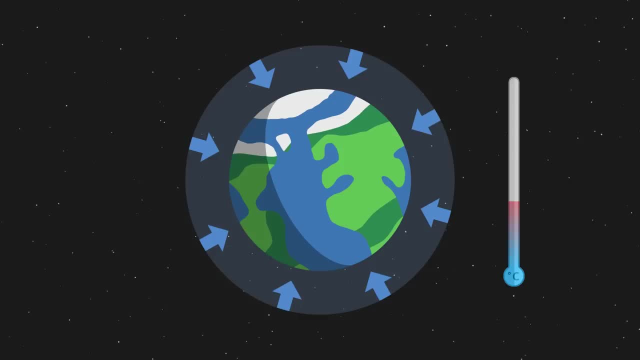 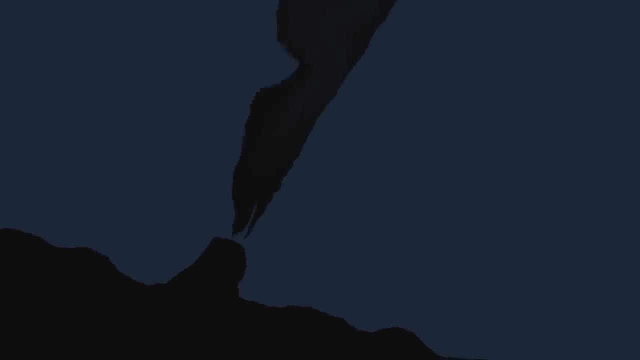 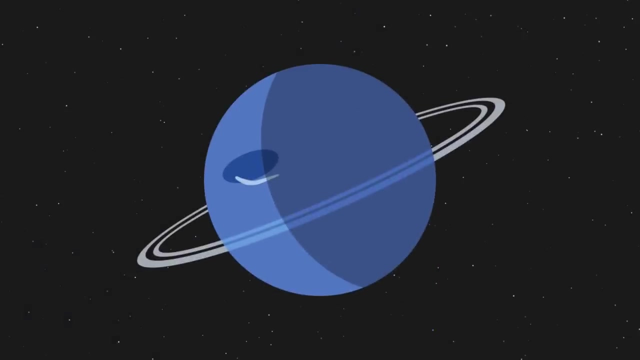 fluids to exist in a natural form. only small quantities can be found at the bottom of the ocean within hydrothermal vents, where temperature and pressure are extreme. although rare on earth, supercritical fluids are relatively common in the universe, especially inside gaseous planets. within their atmospheres, the conditions are so extreme that some layers are actually 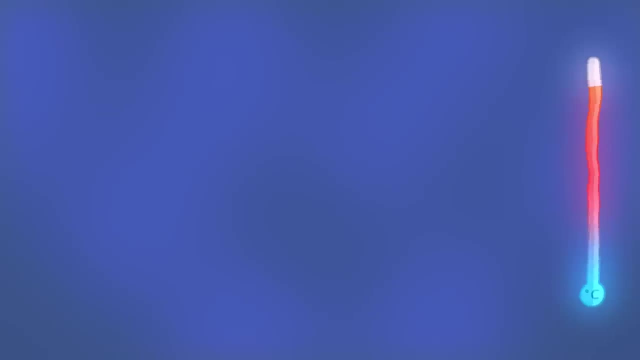 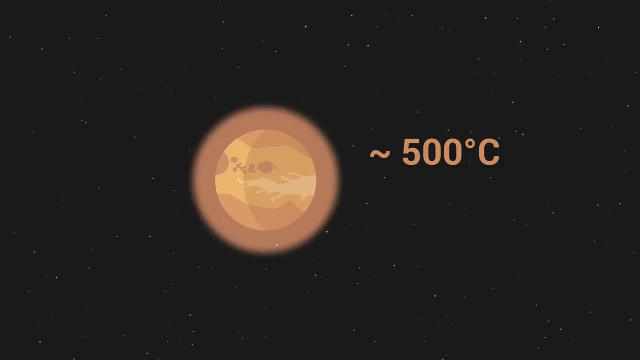 supercritical. similarly, the very hot and thick atmosphere of venus can reach five hundred feet below the same temperature in the advance reinstalling인데atorsindchiediphanos😭. 100 degrees Celsius and a pressure a hundred times greater than on Earth.